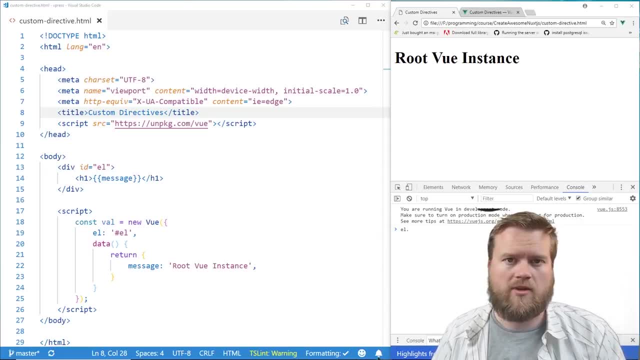 html element. So this could be useful in the future. especially when you get more complicated Vuejs applications, you might find something that you want to do with HTML that would be useful for a directive. So there is a lot to directives, but I'm going to go and show. you just some basics of getting started. All right, so I've got my home and we're going to go ahead and start offering the directives, All right? well, we've been showing them a couple times now and I've got it saved back. 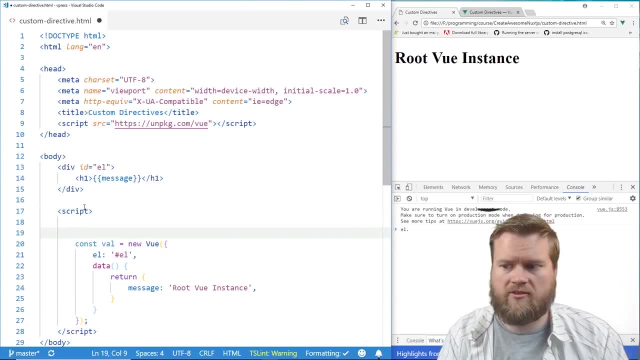 So inside our script tag we can create a directive by just simply typing in View dot directive. so let me do that view capital of you directive and Then you type in the name of it. so I'm gonna create one called colorful and It's an object and 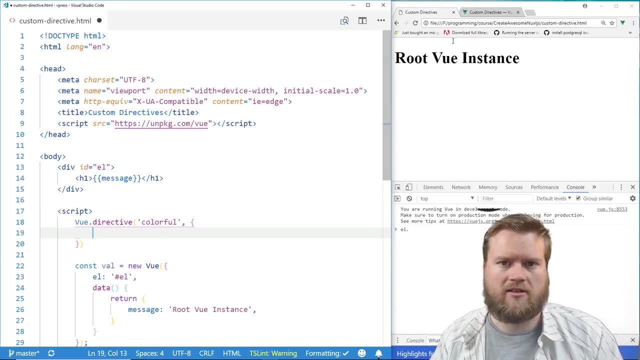 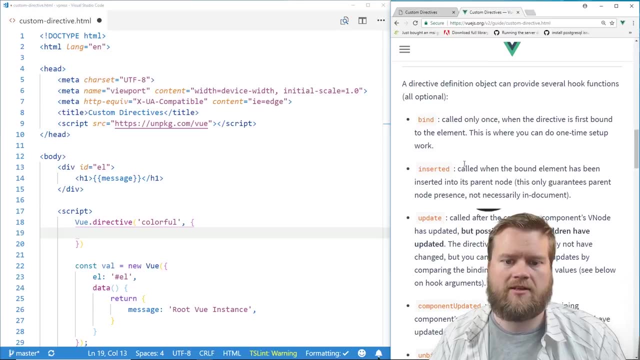 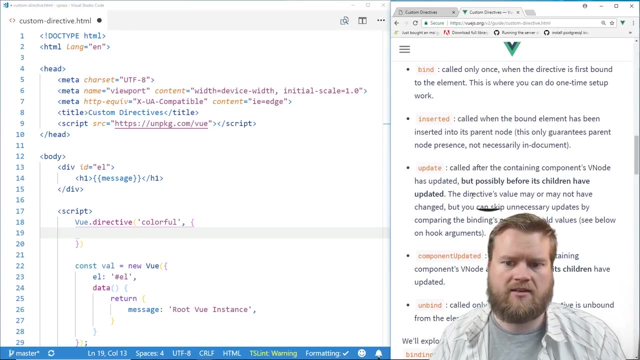 Then you have all these different hooks. They're called hooks and I won't go over all of them. but if you look in the official documentation There's bind which is called only once when the directive is first bounded element Inserted. call when the bound element has been inserted into the parent node. update: called after the containing component V node has updated. 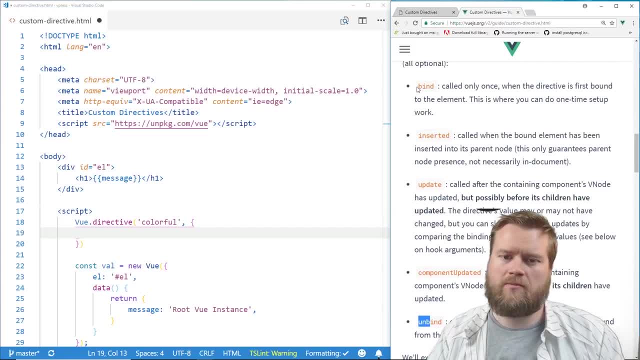 Component updated and unbind. so usually you use most the time you use bind and inserted. I haven't seen too many people use update or component updated, but I'm assuming if you create really complicated Directives you might want to use those. So in our simple example, 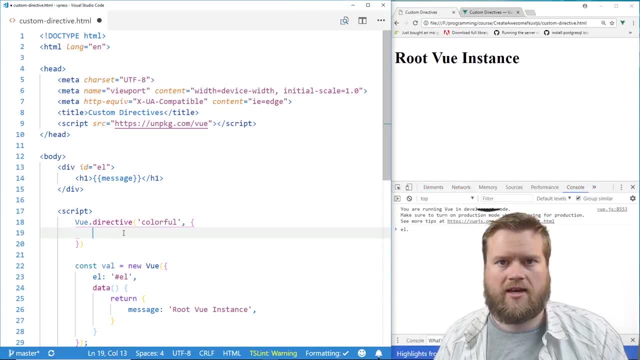 We want to create a directive that we can take a look at Different arguments, how we can pass information to it, And then we want it to just change the color of whatever you attach it to. so it's gonna be really simple. so we're gonna use the inserted and 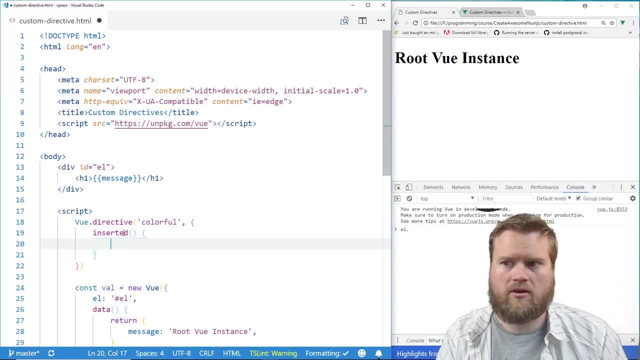 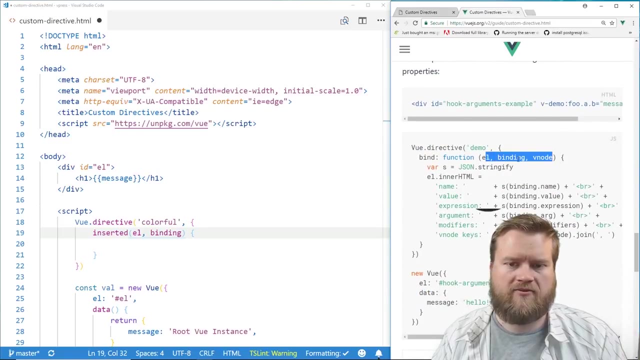 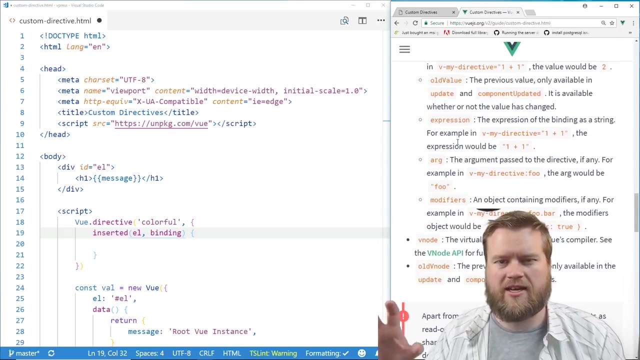 in the inserted Hook we're calling it. it actually has a couple of arguments. it has three as El and Binding and it has one more for V node. You can see here It has El, binding and V node from the official documentation. We're not going to use a V node but you can certainly do that. That's a little bit more complicated. Those are like the nodes that. 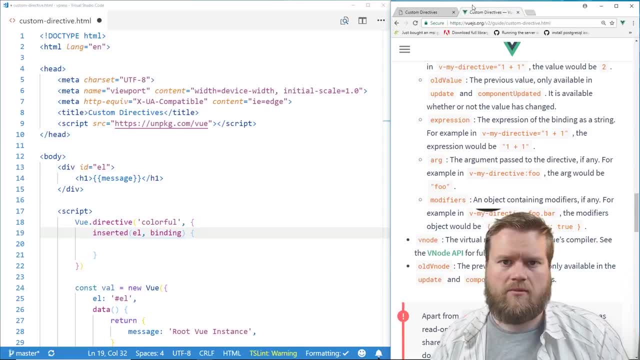 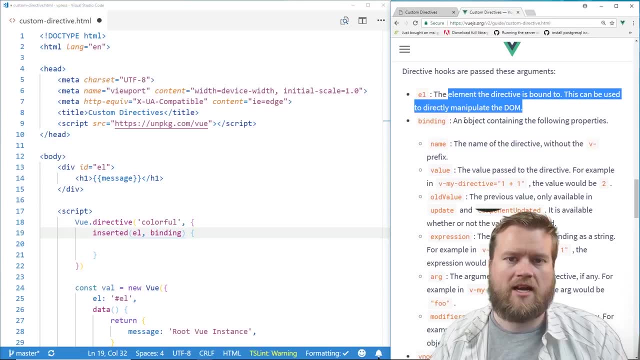 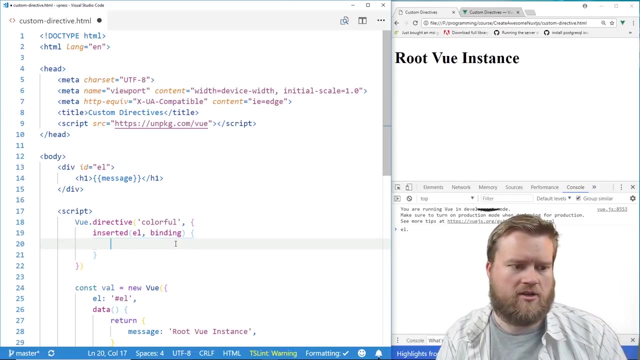 create Your Vuejs application. but El stands for the element. you can see, right here is the element that directive is bound to, and then the binding has a lot of Useful keys in it that we'll take a look at. So we're gonna have El binding here, and for right now I'll just show you well. 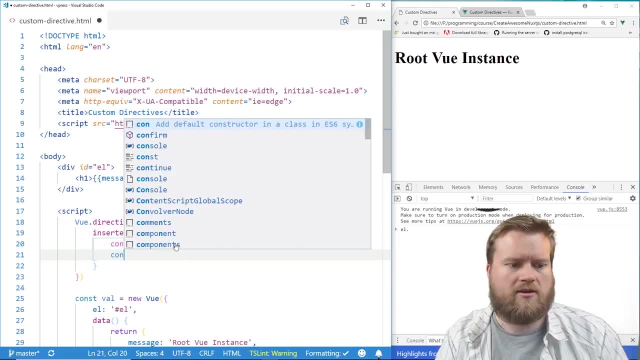 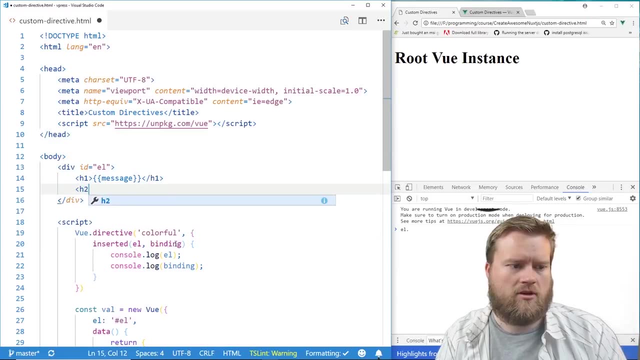 They're gonna consolelog El and we're gonna consolelog binding, Just to show how it works. So let's go and add it to One of our elements and I'll say: hi, This is attached to a new directive, custom directive. Okay, so if we go back to start now, we can add it to it now, just like. 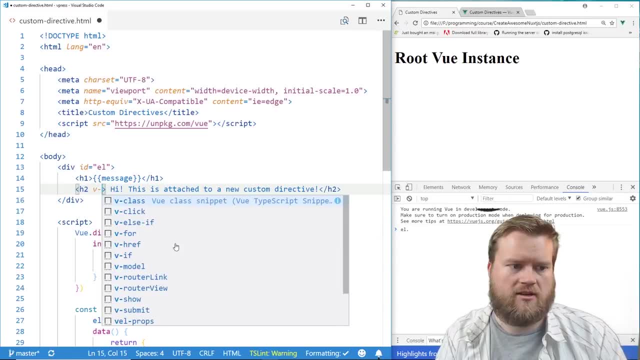 like every other directive, you start with V dash and then you type in the name: we're gonna call it Colorful because that's the name we called it here. And first I'll just put in an argument. You can actually put in arguments by putting dot. 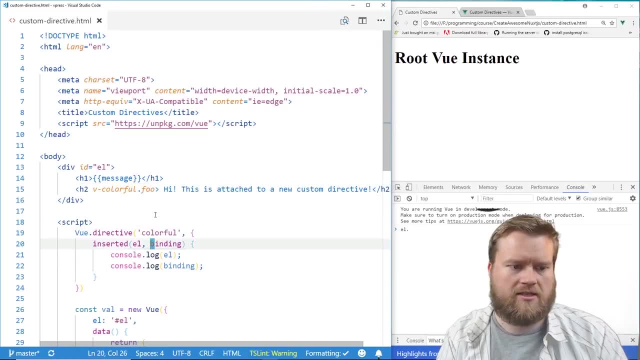 We'll do dot foo and we'll see what that looks like here. So I'm just going to refresh it, Say hey, hi, this is attached to a new custom directive and we're gonna look at the bottom here. so I'm gonna kind of get out of the way. 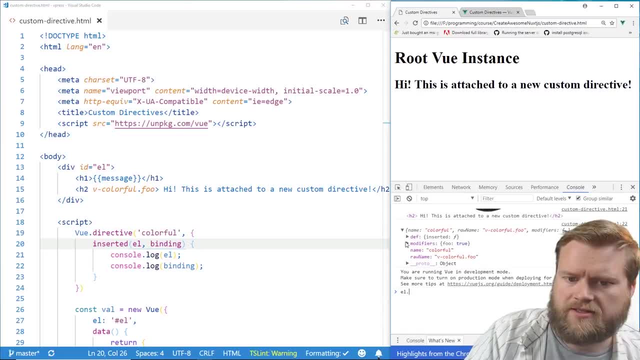 And in the bottom you see there's modifiers. So obviously EL is the element hi. this is attached to the new custom directive. But you can see right here is the actual binding. So you get the name, which is Colorful. 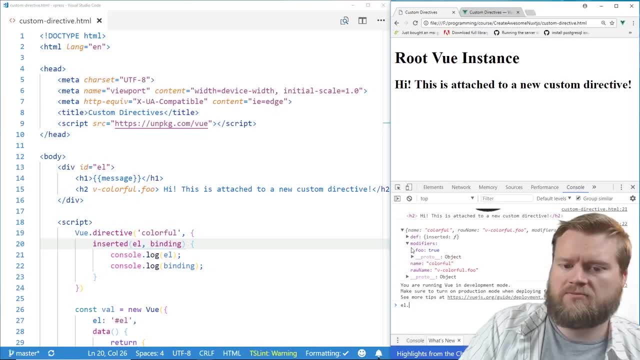 We get the raw name, which is the complete name, And we have these modifiers, which has foo, which is true, But if we go to definition, it tells you that we have it inserted in here. so it's kind of a lot of neat stuff. 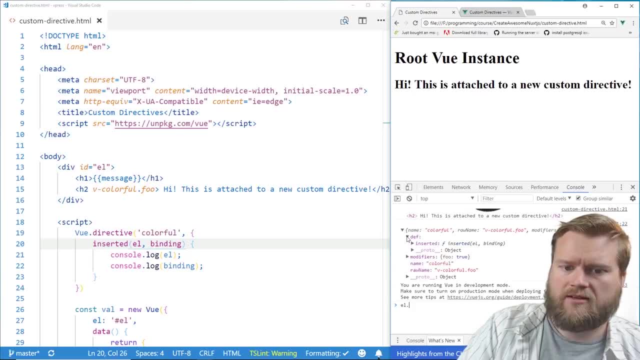 that you might need to look at. So let's take a look. and it's inserted. We have some more information here. modifiers: We have foo equals, true, So that's helpful. So let's take a look at how we would use this. 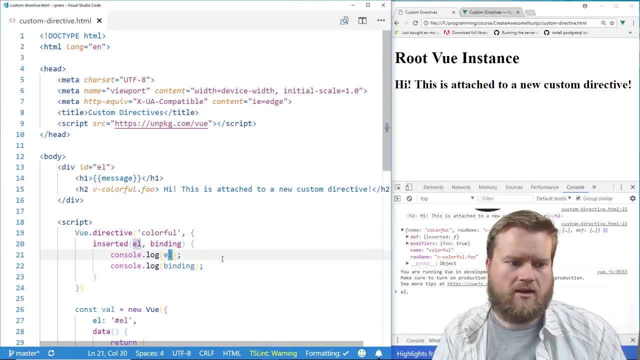 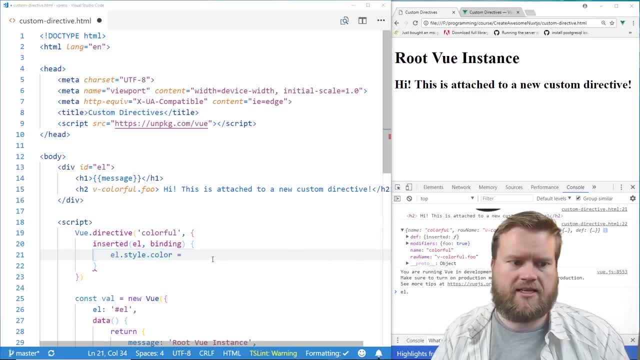 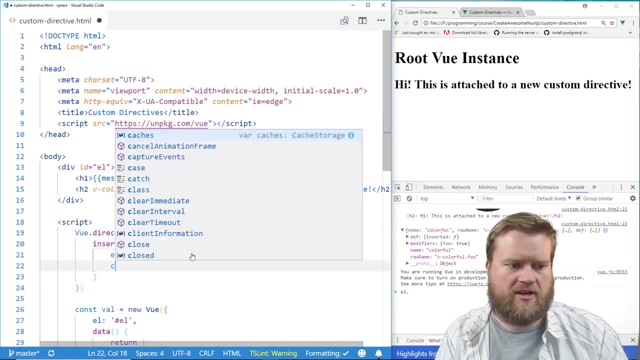 And I'm gonna put the style, And I'm gonna put the style, And that's gonna equal our bindingvalue. So we're gonna actually have a value attached to this And we'll take a look at what it looks like when we have a value. 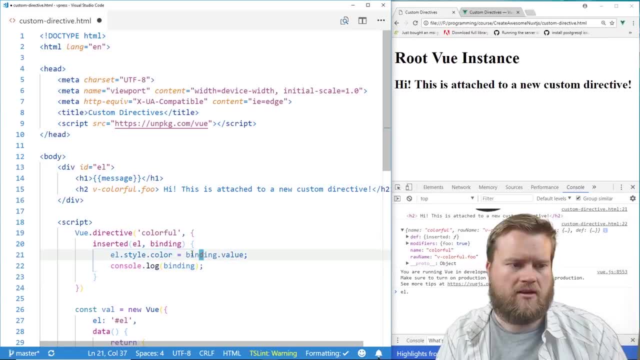 So we're gonna consolelog binding again And to add a value to it we just simply put in an equal sign and then quotes. Now, if we just put a value in here like red, it's gonna give us an error. 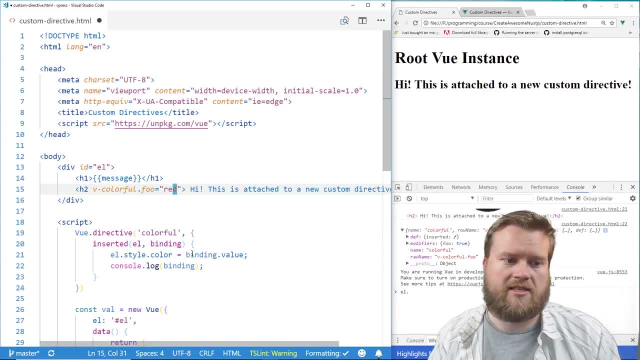 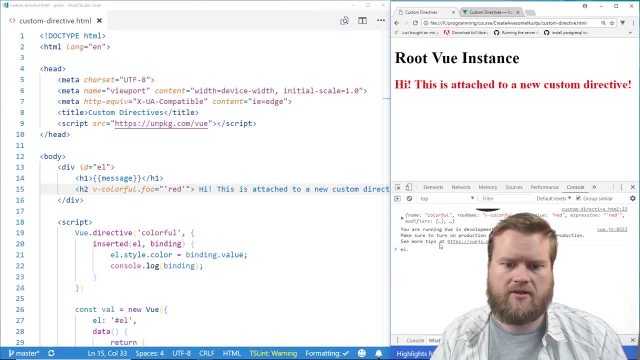 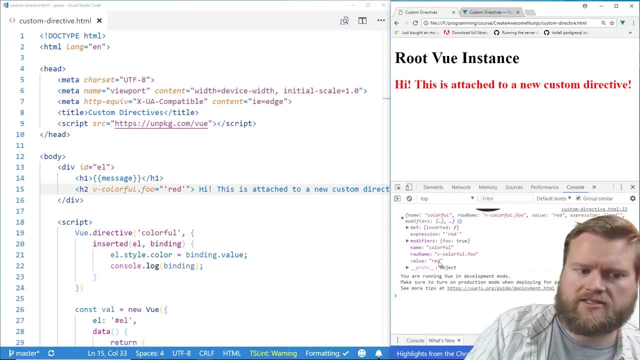 because it expects this actually a property. that's inside our view instance, but if we put it in single quotes then it's actually a string. so we do this. now we can see we have our name colorful and we have a value of red. so that's exactly what we want and you can. 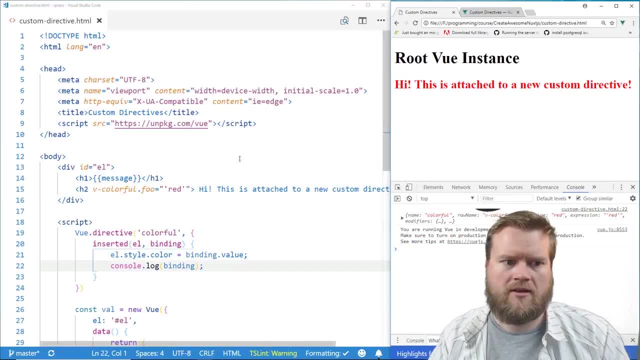 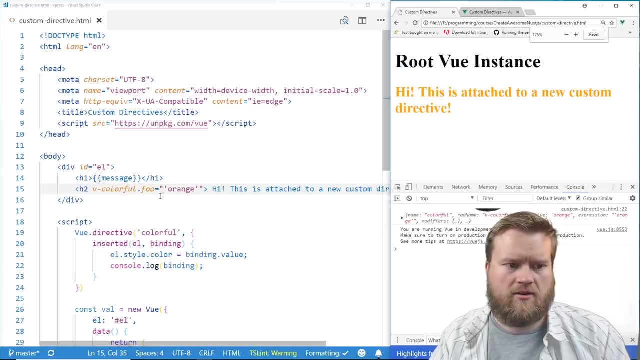 see here it turned red, so we know it's working. so let's say: we add in orange here and we save it. now it's orange, or we can do blue, blue here, and we could say, we can even do this red. so we'll say: if binding dot and we could see here, we 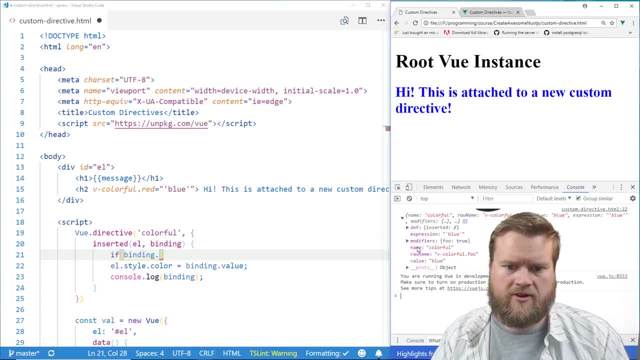 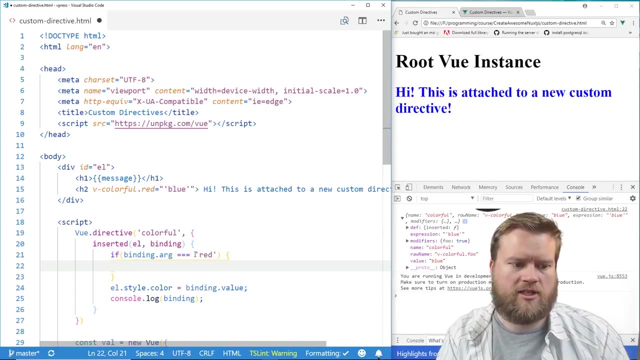 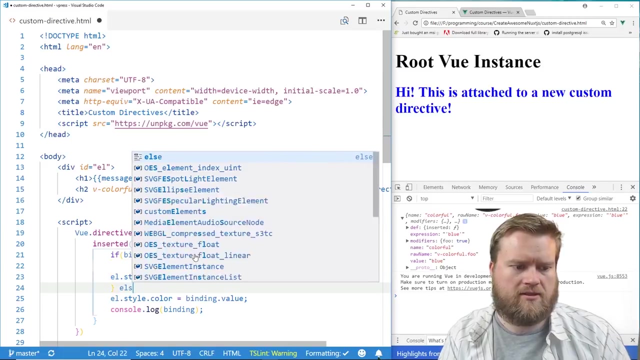 have an expression and we have our name and we have our name and we have our name, our raw name and value. if we do binding that arg say equal, equal, equal red, then we'll change the style, the red, else we'll change it to whatever's in here. 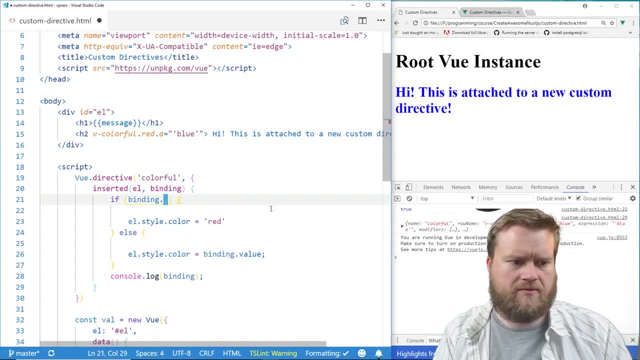 this is actually supposed to be so. we do binding dot modifiers, dot red, and that'll either turn true or false. so if it's true, turns red, but it let's say we put this to orange, it's blue. so so you can do modifiers too. that's another way of adding a little bit more complexity to.